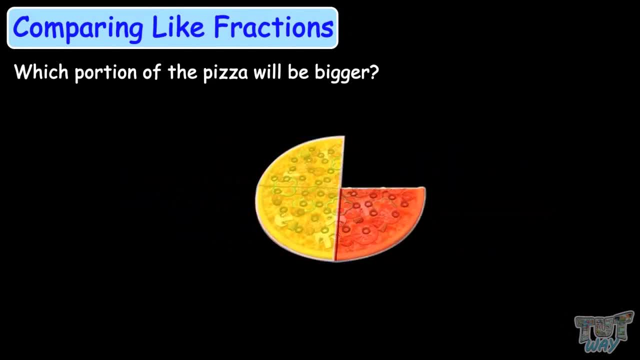 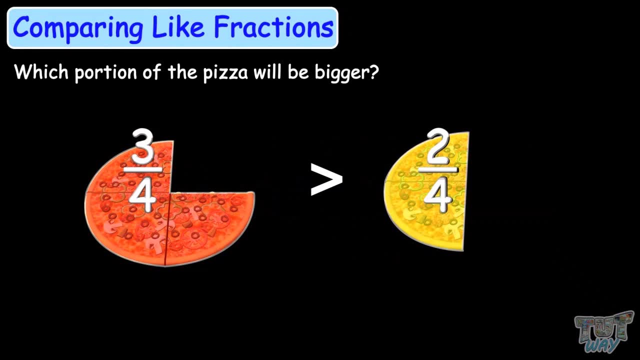 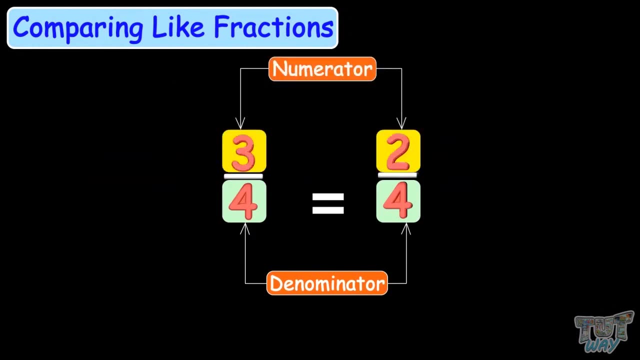 You can visually compare that 3 fourth pizza is bigger than 2 by 4 pizza. From this example, you also learn that if the denominators are same, you just need to compare the numerators for comparison. This is why 2 by 4 is smaller than 3 by 4.. 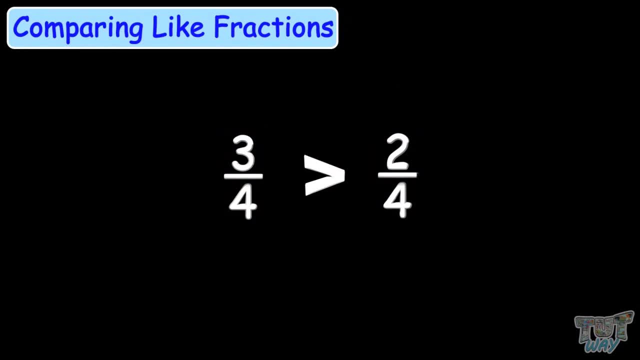 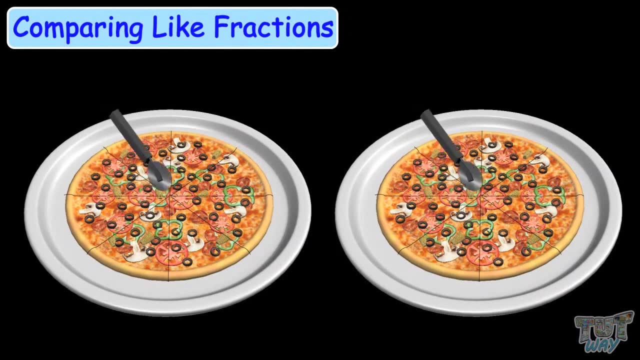 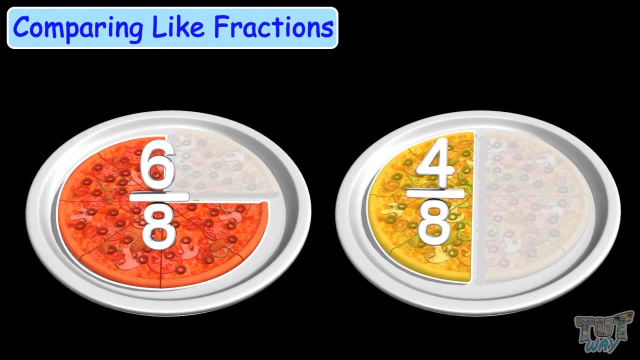 Here we have another example. Your mom cooks a pizza and cuts the pizza into 8 equal parts, and she will either give you 6 eighth pizza or 4 eighth pizza Now, in which case you will get more pizza. This is 4 eighth portion of the pizza. 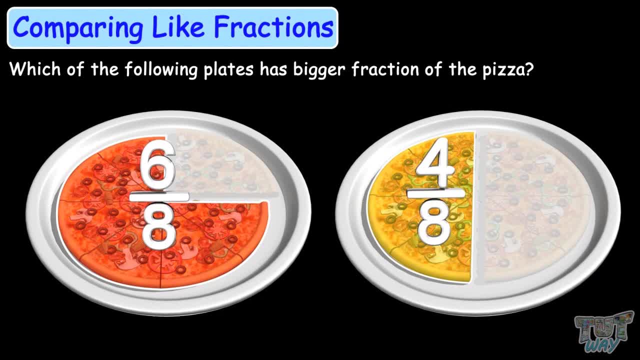 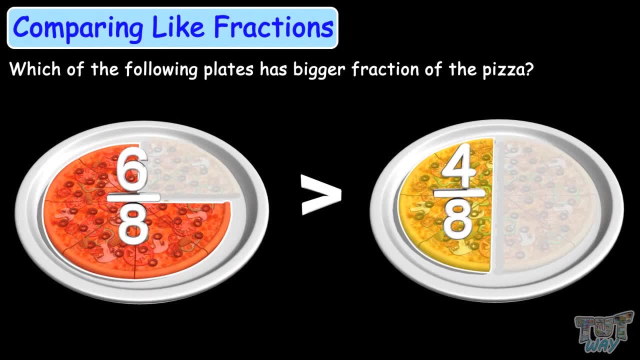 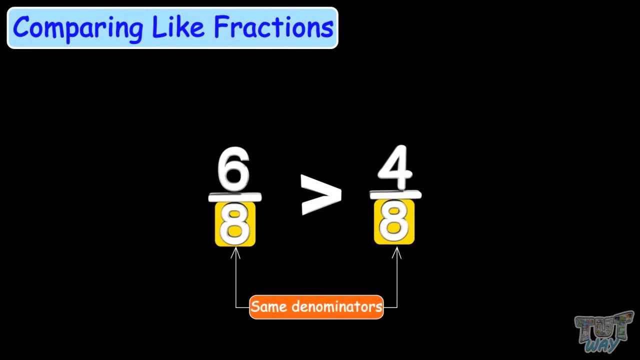 Now again, you can visually compare that 6 eighth pizza is more than 4 eighth pizza. You can also notice that these are like fractions, that is, having same denominators. So you just need to compare the numerators to compare the fractions. 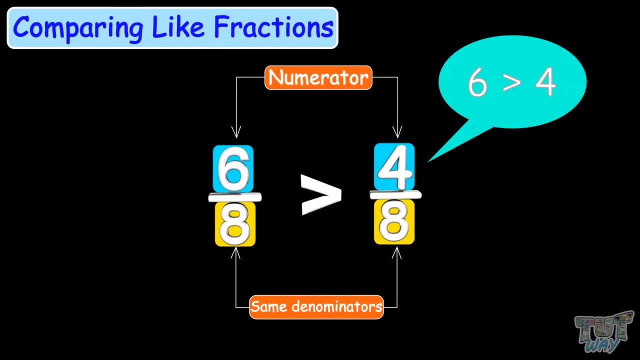 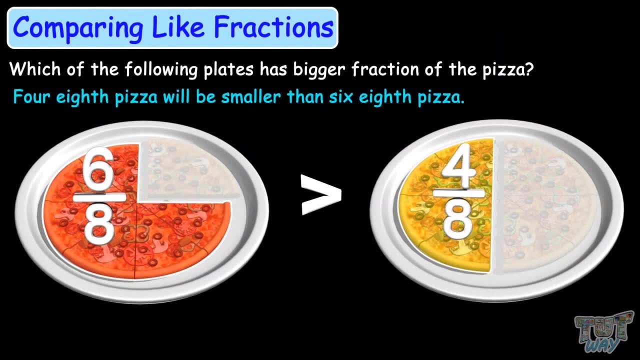 4 is smaller than 6.. So 4 by 8 is smaller than 6 by 8.. So 4 eighth of the pizza will be smaller than 6 eighths of the same pizza. Now let's compare more like fractions in a quick fashion. 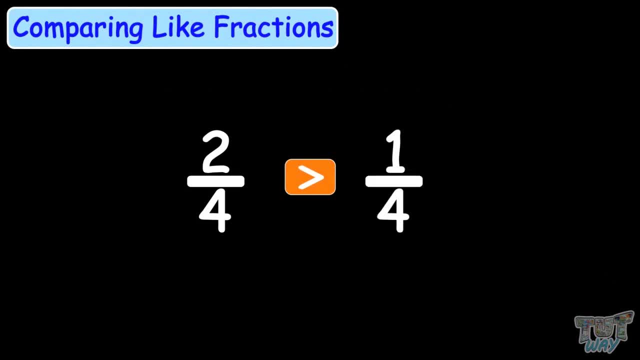 2 by 4 is greater than 1 by 4.. 3 by 4 is greater than 2 by 4.. 1 by 3 is less than 2 by 3.. 7 by 8 is greater than 3 by 8.. 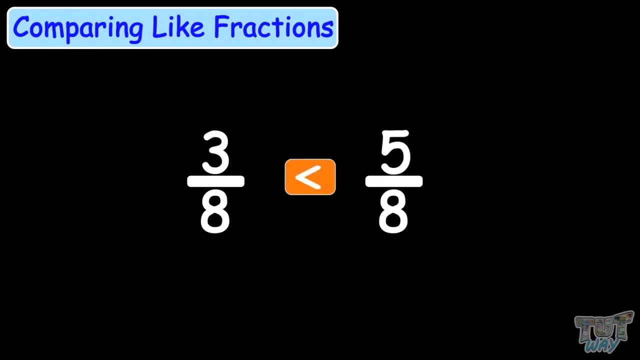 3 by 8 is less than 5 by 8.. 1 by 8 is less than 4 by 8.. So all these are like fractions, that is, having the same denominator, And when we are comparing like fractions, we only compare numerators. 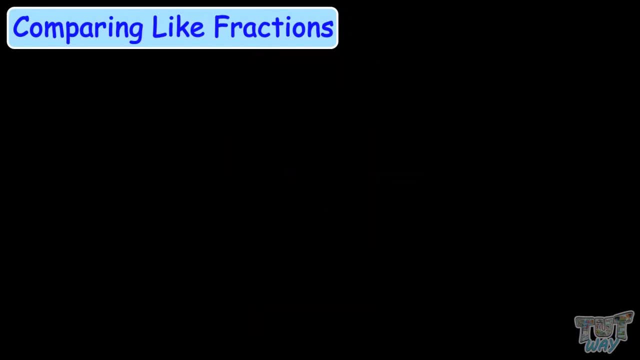 Here we have more examples: 7 by 12 is greater than 2 by 12.. 9 by 12 is greater than 7 by 12.. 2 by 12 is greater than 1 by 12.. 3 by 12 is less than 9 by 12.. 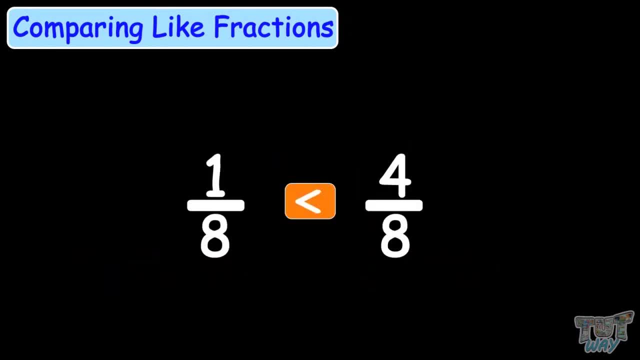 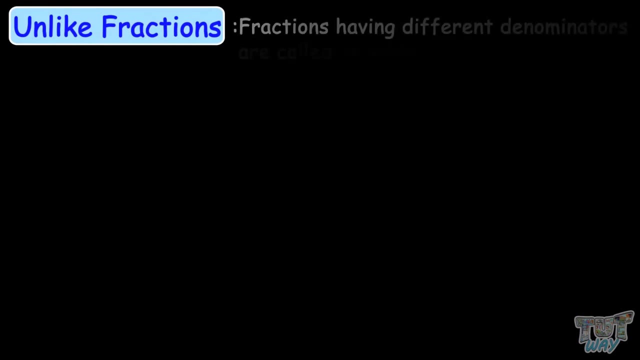 Now you know how we compare like fractions and why we only need to compare numerators while comparing like fractions. Now we will see comparing unlike fractions. Fractions having different denominators are called as unlike fractions- 3 by 4 and 5 by 6.. 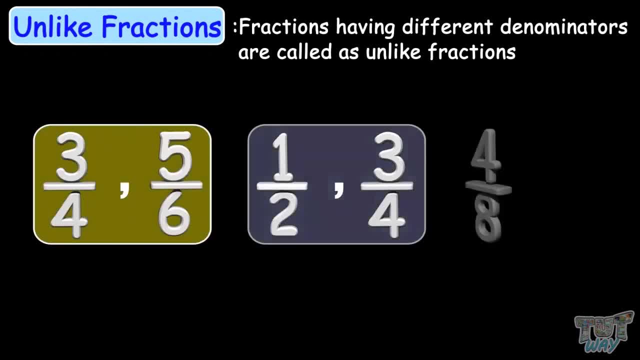 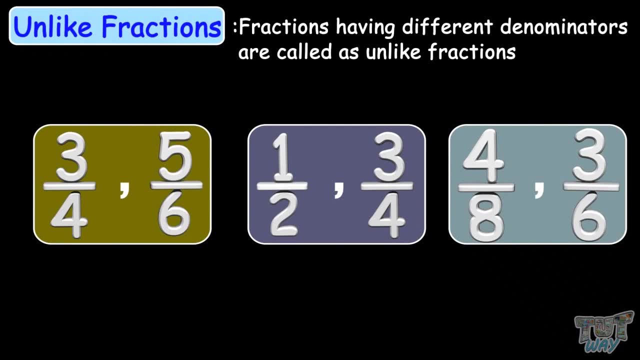 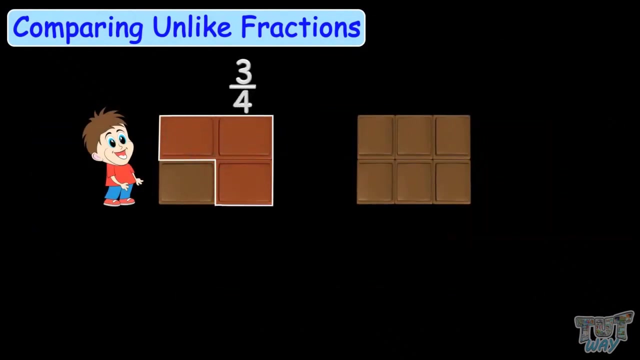 1 by 2 and 3 by 4.. 4 by 8 and 3 by 6.. These are examples of pairs of unlike fractions because they are having different denominators. Now let's see how we can compare them. One child has been given 3 fourths of a chocolate. 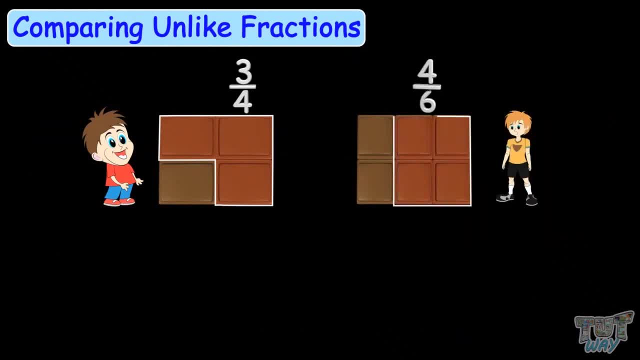 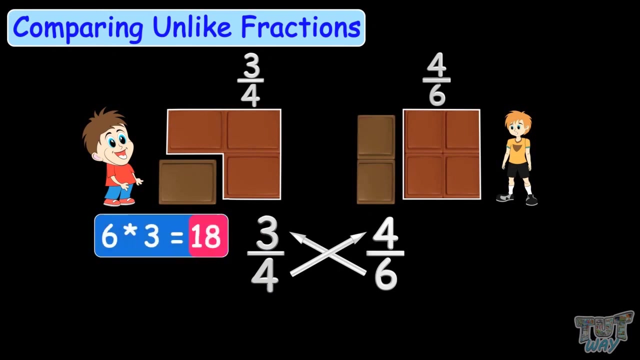 And one child is given with 4 sixths of the same size chocolate. Now who got more? Take the two fractions to be compared and multiply the denominator of the one with the numerator Like this: Multiply 6 by 3.. Write the product here. 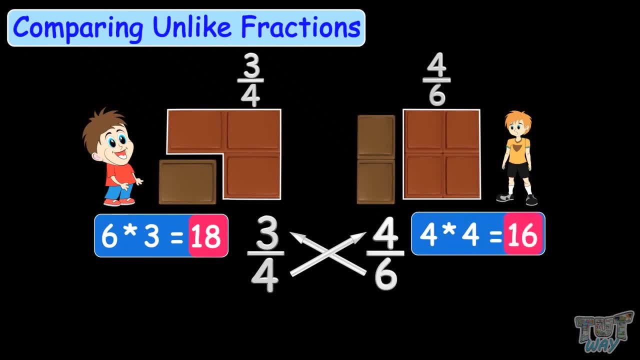 Multiply 4 by 4.. And write the product here. You get the bigger product. that is 18 on this side. That is 3 by 4.. So this fraction is bigger. 3 by 4 is bigger than 4 by 6.. 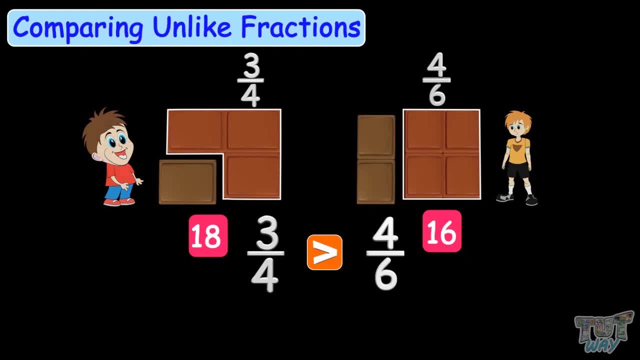 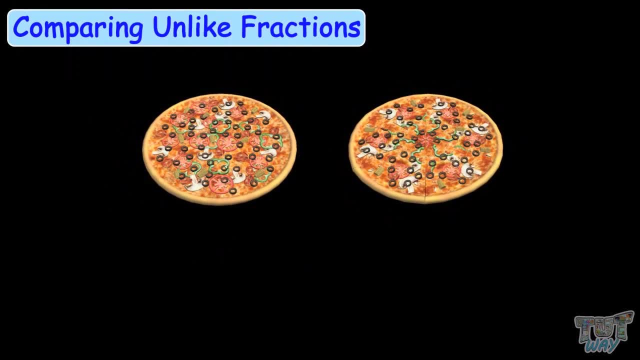 Here we have another example. We have two pizzas of the same size And we cut one into 8 slices And the other one into 6 slices. Now if we take two pieces from this pizza, That is 2 by 8.. 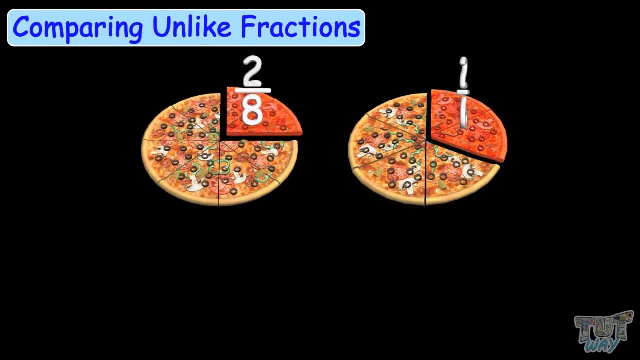 And we also take two pieces from this pizza. That is 2 by 6.. Now which fraction is bigger, 2 by 8 or 2 by 6?? Write the two fractions side by side And multiply the denominator of the one with the numerator of the other. 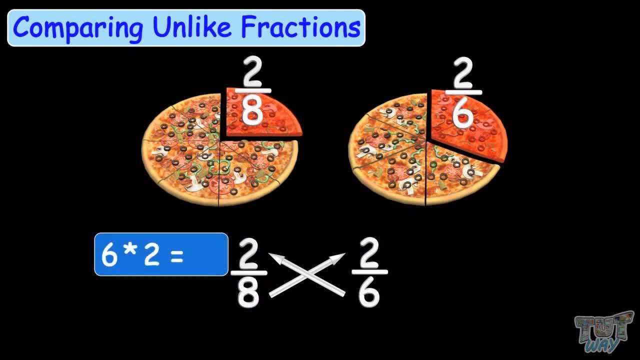 Multiply 6 by 2. And you get 12 on this side. Multiply 8 by 2. And you get 16 on this side. So we get a bigger number on this side. So 2 by 6 is bigger than 2 by 8.. 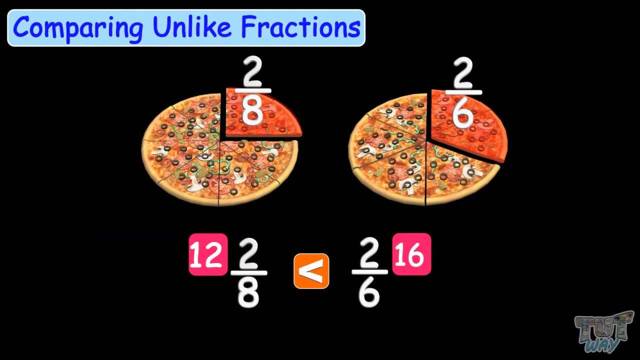 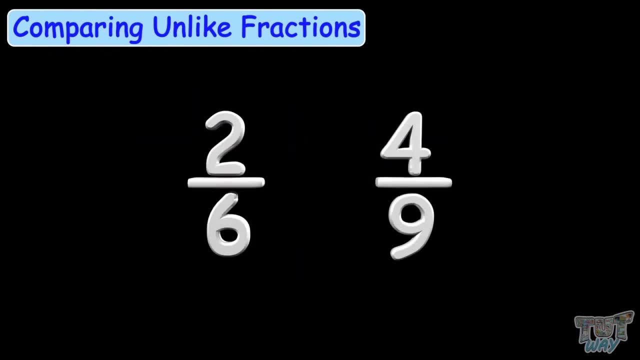 Now let's compare some unlike fractions in a quick fashion, Comparing 2 by 6 and 4 by 9.. 6 multiplied by 4 is 24.. 9 multiplied by 2 is 18.. So we get a bigger number on this side. 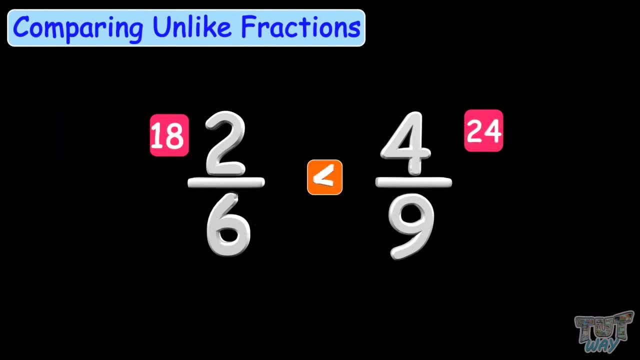 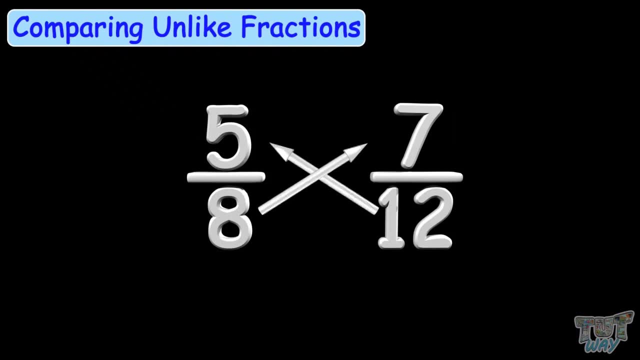 So 4 by 9 is a bigger fraction. Now let's compare 5 by 8 and 7 by 12.. 8 multiplied by 7 equals 56.. 12 multiplied by 5 equals 60. We get bigger number on this side. 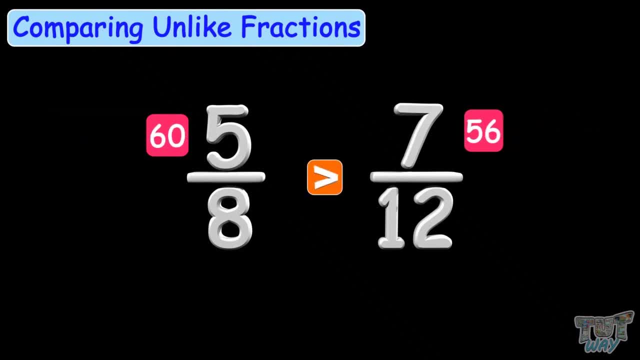 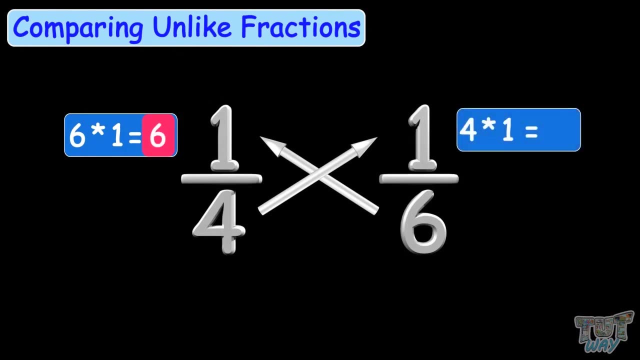 So 5 by 8 is bigger fraction. Now let's compare 1 by 4 and 1 by 6.. 6 multiplied by 1 equals 6. And 4 multiplied by 1 equals 4.. And 6 is bigger than 4.. 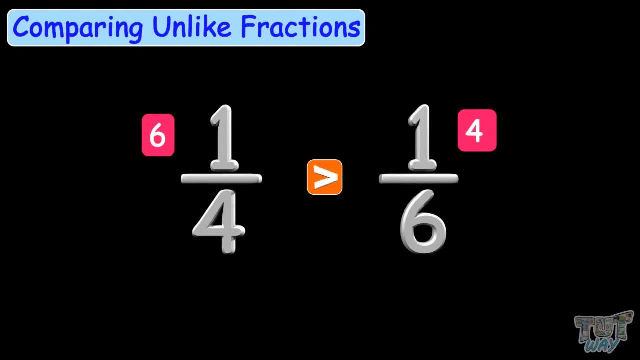 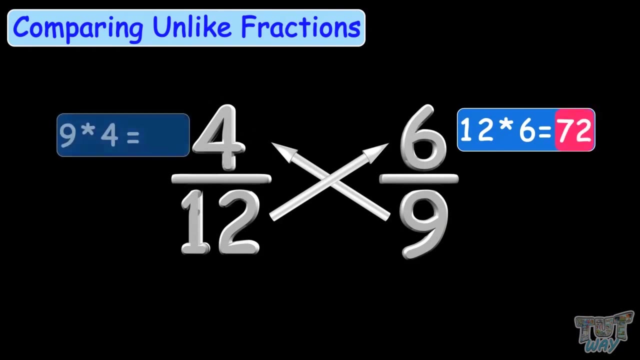 So 1 by 4 is a bigger fraction. Here we have another pair of unlike fractions: 4 by 12 and 6 by 9.. 12 multiplied by 6 equals 72.. And 9 multiplied by 4 equals 36.. 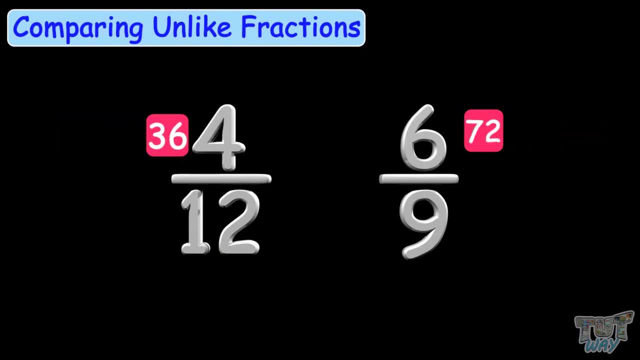 You got a bigger product on this side. So 6 by 9 is a bigger fraction out of these two unlike fractions. So, friends, now we know how to compare unlike fractions. Now we will learn how to compare mixed fractions. 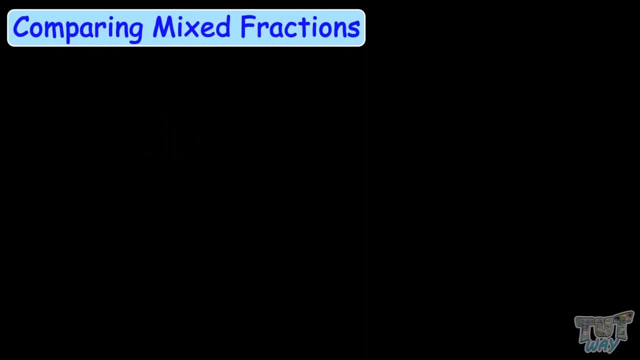 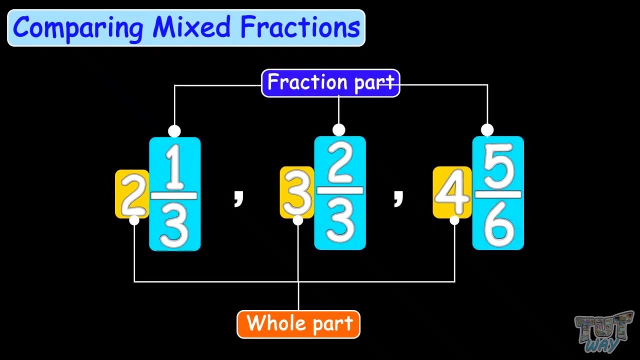 Here we have some mixed fractions: 2, 1 by 3.. 3, 2 by 3.. 4, 5 by 6.. They have a whole part and a fraction part. Now let's see how we can compare these. 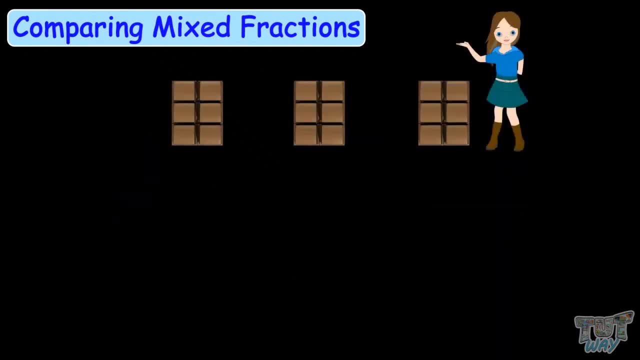 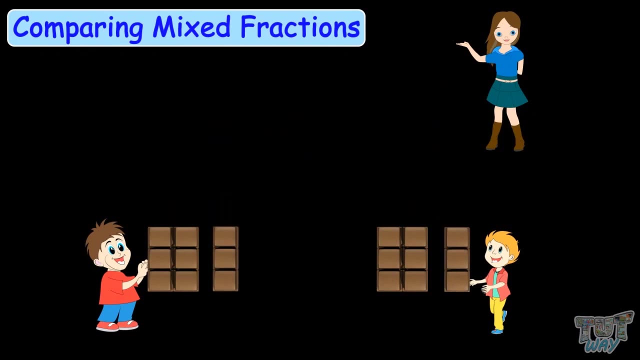 I have three chocolates. I have to distribute them between two children. So I will give one chocolate to each child And then we'll give a half chocolate to each child. So each child's share is 1, 1 by 2.. 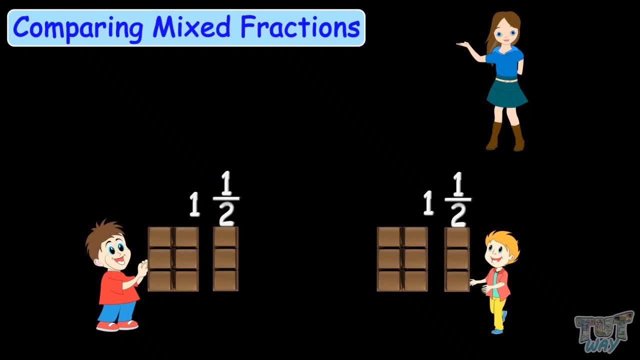 So these are mixed fractions or mixed numbers. They are having a whole part- 1- and a fraction part, 1 by 2.. And these mixed numbers are equal. They are having the same whole part as well as same fraction part. 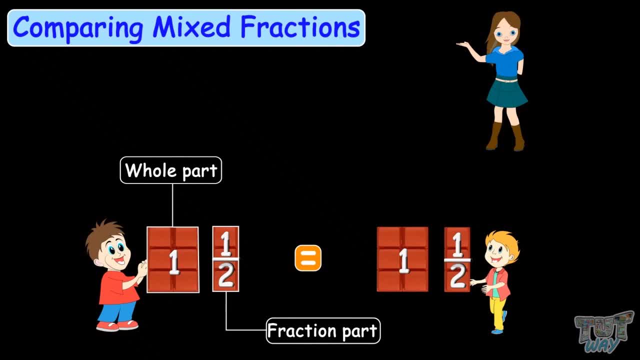 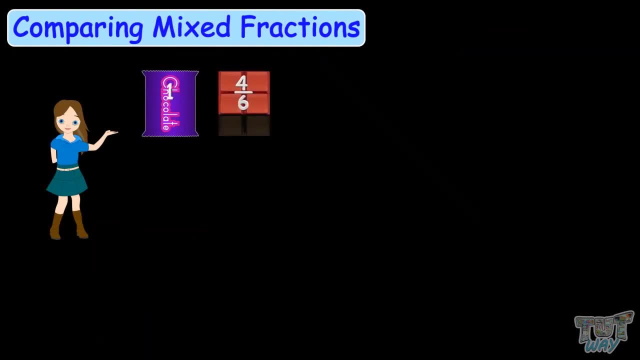 Now let's have another example. Tia is having one whole chocolate And also a 4, 6 chocolate. Sam is having one whole chocolate And also a 2, 6 chocolate. Now who has a bigger share of chocolate? 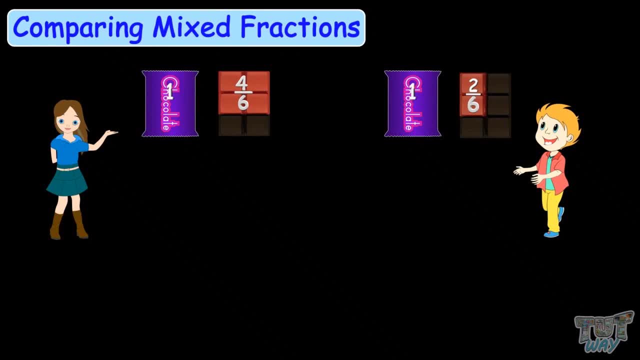 Here comes a comparison of mixed fractions. One child is having one 4 by 6 chocolate And the second child is having one 2 by 6 chocolate. For comparing mixed fractions we first compare the whole parts. In our example, whole parts are equal. 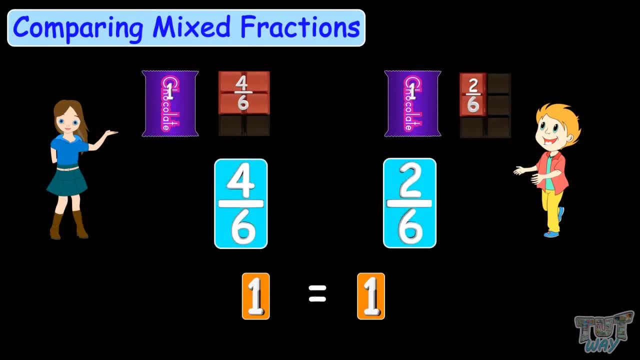 So we will now compare the fraction parts. The fraction parts are having same denominators, So they are like fractions. And we know we compare only the numerators for comparing like fractions. So 4 by 6 is bigger than 2 by 6.. 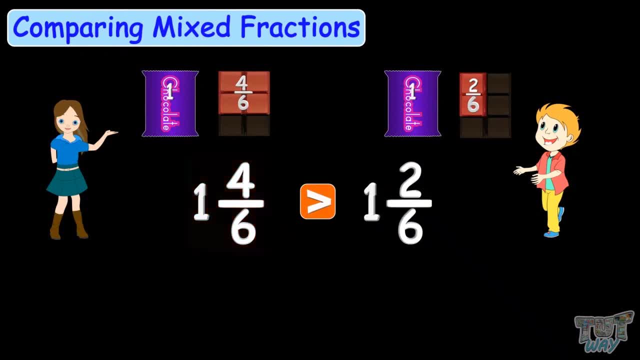 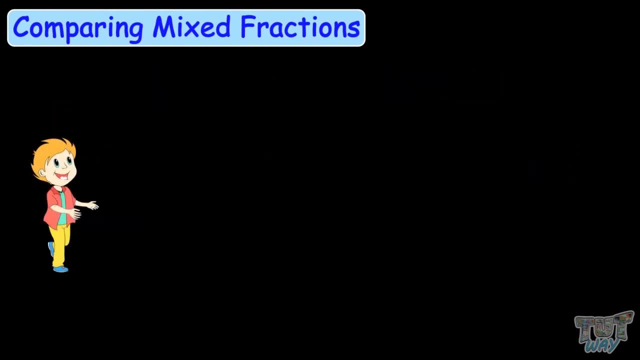 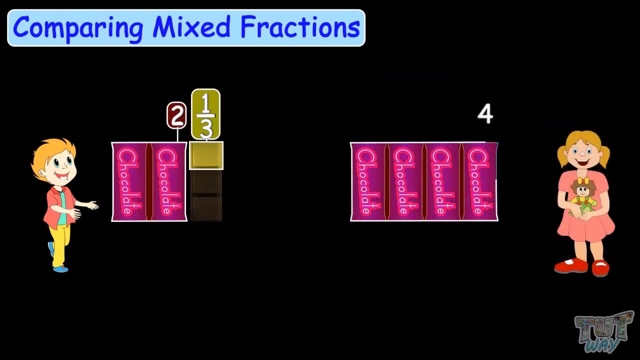 Hence 1, 4 by 6 is a bigger fraction. Now let's compare more mixed fractions: Sam has 2 whole chocolates And 1 third chocolate also. Olivia has 4 whole chocolates And a 2 third chocolate also. 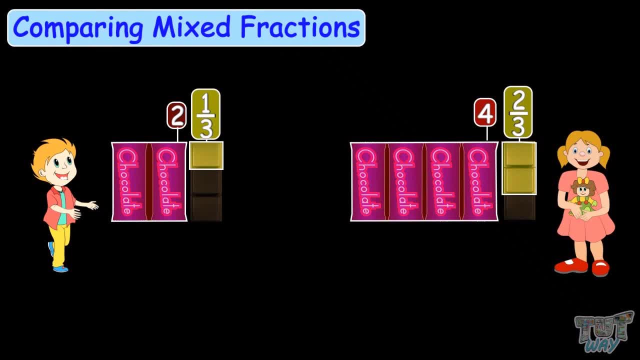 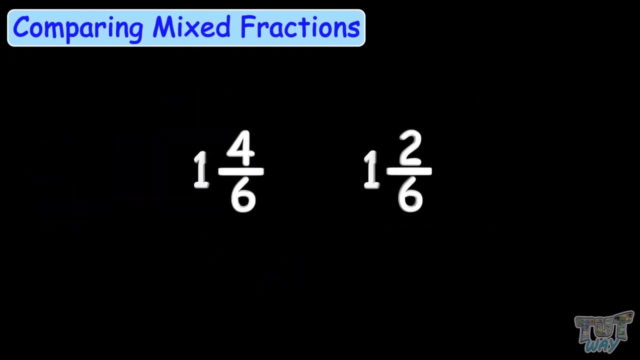 Who got more chocolates. You can judge that the child with more number of whole chocolates has more chocolates. So no need to compare the fraction part. So now we have learnt: for comparing mixed fractions or mixed numbers, We first compare the whole parts. 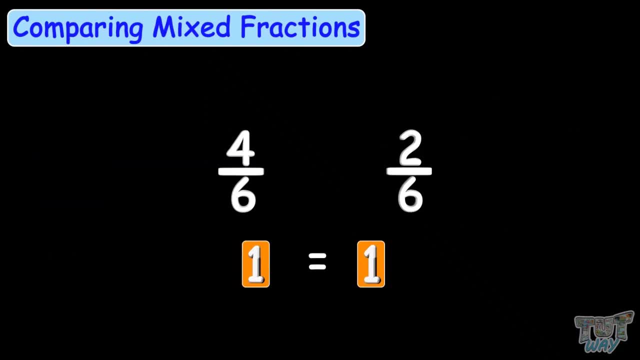 And if whole parts are same, then only we compare the fraction portions. Now let's have some more comparisons. Which of the following mixed number is bigger? The one with the bigger whole number. So this mixed fraction is bigger. Now, which of these mixed fractions is bigger? 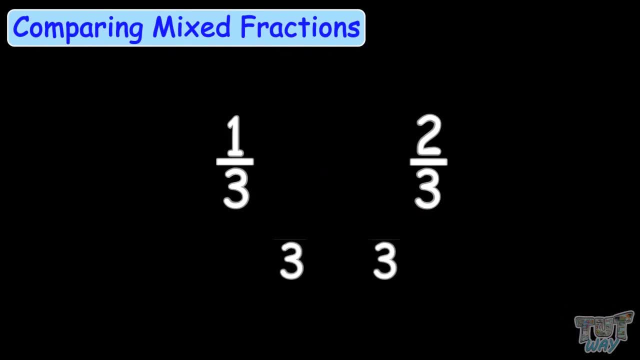 Again, the fraction with a bigger whole number should be bigger. The whole parts are same here, So we will be comparing the fraction portions 1 by 3,, 2 by 3.. These are like fractions, So we will just compare the numerators. 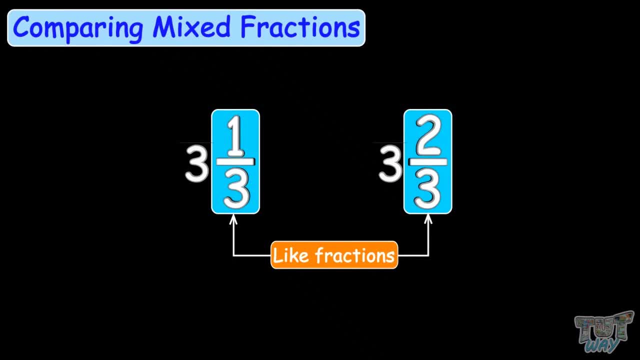 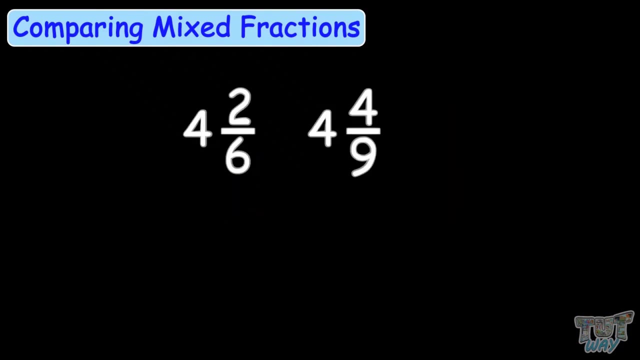 for comparing these fractions: 2 is bigger than 1.. So 2 by 3 is bigger than 1 by 3.. So this mixed number is a bigger number. Now, which of these mixed numbers is bigger? 4, 2 by 6.. 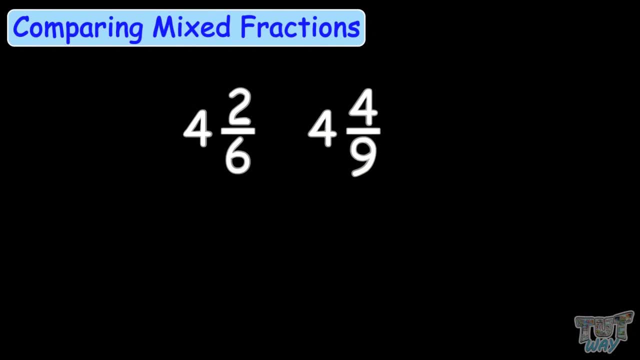 4,, 4 by 9.. Again, the whole parts are same. So we will compare the fraction portions. But the fraction portions are unlike fractions. Both are having different denominator. So we have already learnt how to compare unlike fractions.